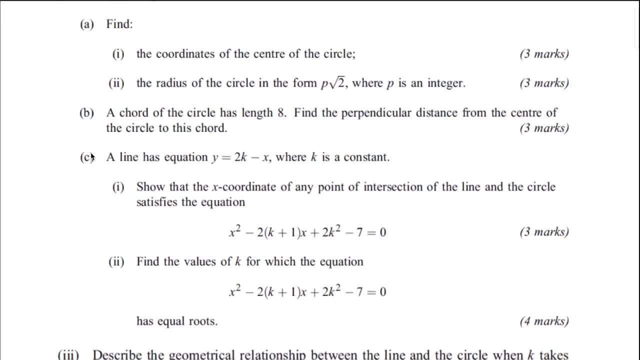 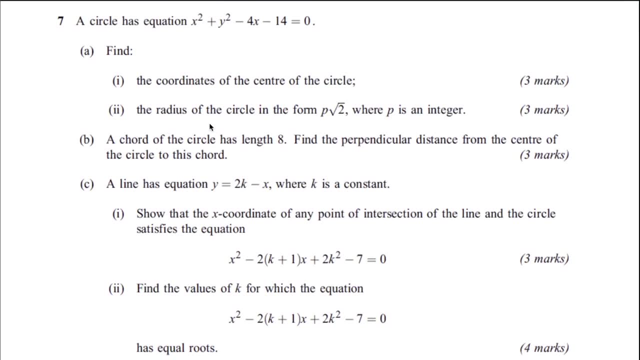 a third part to part C, but most of the question is here on the screen. Please have a go and then come back and watch the solution. Okay, so the question says a circle has equation: x squared plus y squared, take 4x, take 14, equals 0. and part A says: find the coordinates of the center. 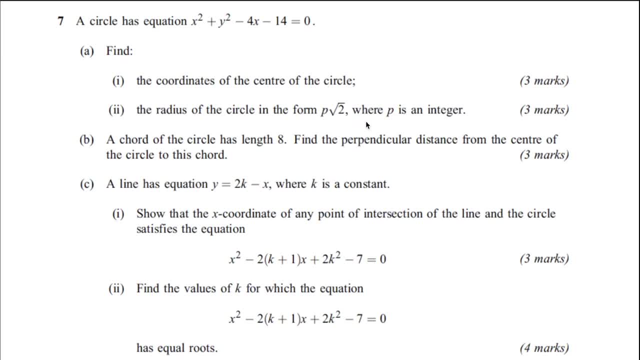 of the circle and the radius of the circle in the form p root 2, where p is an integer. All right. so for this one you need to know the standard form of an equation of a circle which looks like this. So it's x, take a squared plus y, take b squared equals r squared. 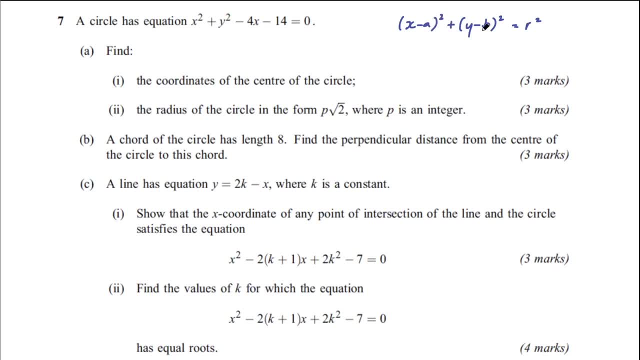 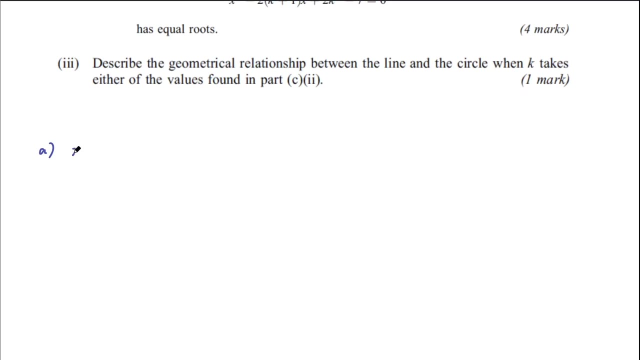 So if we can get it into that form, we'll be able to see the center and find the radius as well. So we'll have to rearrange this equation a little bit and then hopefully we'll be able to get the answer. Okay, so I'm going to write this down below. So for part A we had x squared plus y squared. 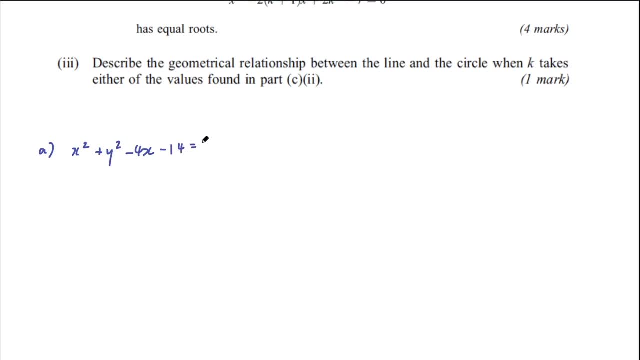 take 4x, take 14, equals 0. and again we want to rearrange it in the form of the standard equation of a circle, So I'll combine those x terms. So we have x squared: take 4x plus y squared: take 14, equals 0. 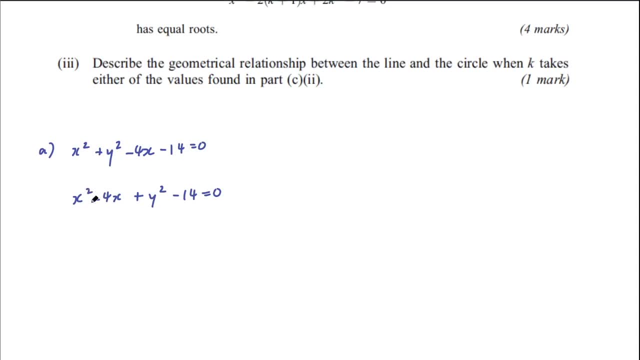 and for this now I want to use completing the square. So I have that x take a constant in brackets, all squared. So to complete the square in this we take half of the coefficient of x and then square it. So x take 2 all squared and then if we expanded that out, we would have an 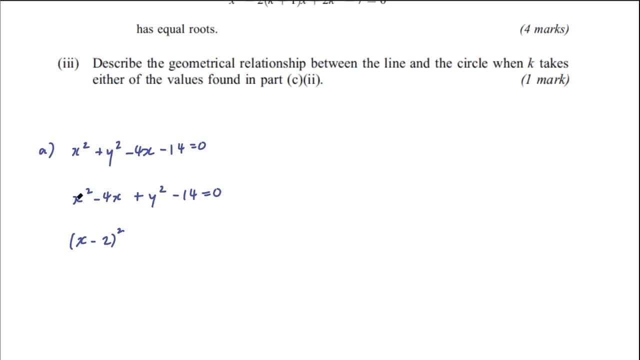 additional plus 4, which we wouldn't have in this equation. So we need to subtract 4 to make up for that fact. So expand that out. you'd have plus 4. take 4, then we would still have the same equation. Then we still have that plus y squared. take 14 equals 0 and combine those constants negative. 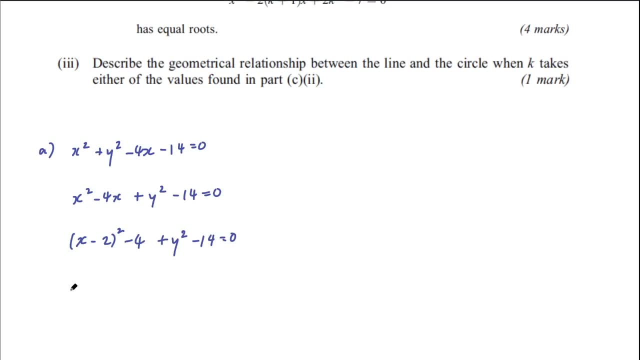 4, take 14 negative 18.. If I add that to the other side we'll have x, take 2, all squared plus y squared equals 18.. So now we have it in the form of the equation of a circle, and here we can say that the center 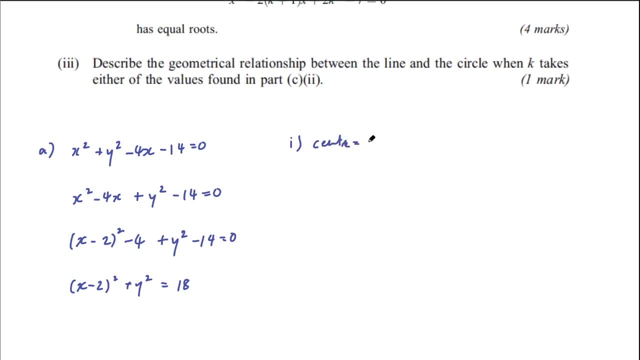 will be now, when you don't have, you know, those brackets with a constant term in it, then the coordinate is 0.. So the y coordinate for this equation is 0. the x coordinate is 2.. So if it's negative 2, then the x coordinate will be a positive 2, and vice versa. So this center here will be 2.. 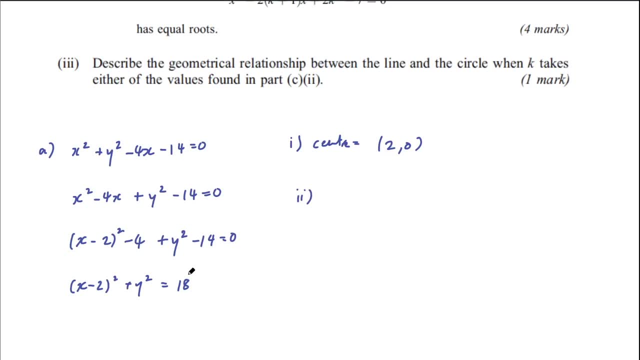 0 and the radius. remember that's the radius squared. So the radius will be 8, the square root of 18. and then, if we simplify that third, this is like 9 times 2. So the square root of 9 is 3.. 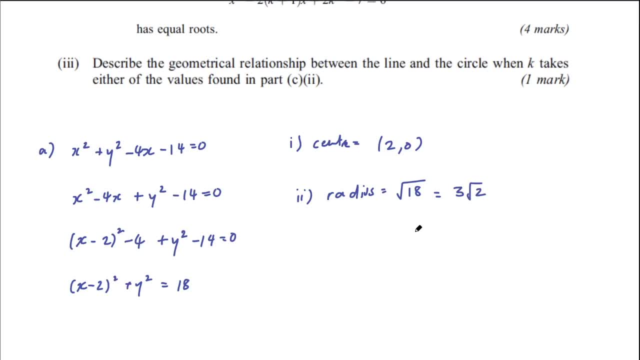 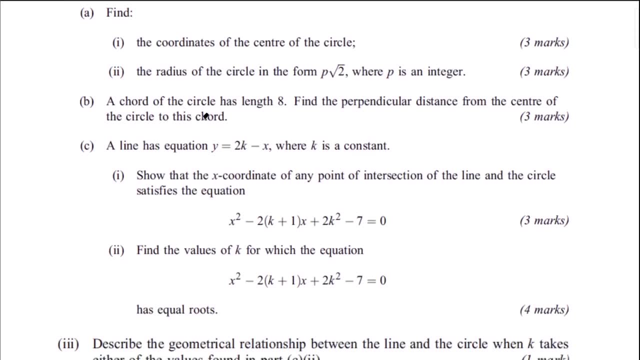 So we could write that as 3 square root 2.. Okay, so that's in the form: p root 2.. Okay, so that's part 1 and 2.. Part b says a chord of the circle has length 8.. Find the perpendicular distance. 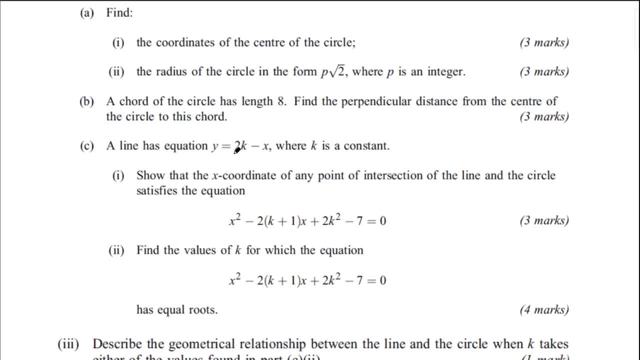 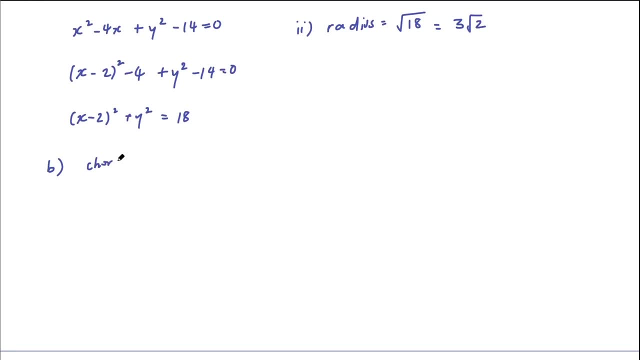 from the center of the circle to the chord. Alright, so there is a standard way of doing this. So for part b we have a chord length of 8., 8 units. they don't give us any specific units, So to find the distance from the center to the chord we use basically Pythagoras. So we can say: 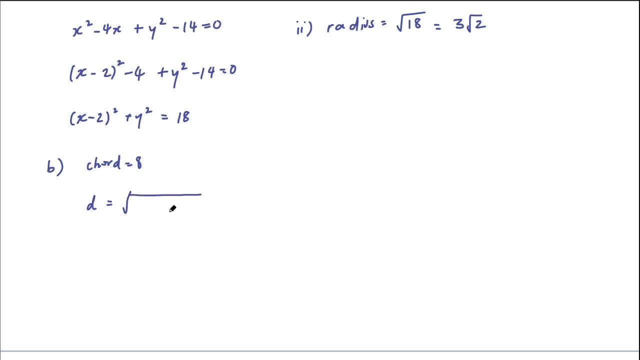 the distance equals the square root of the radius squared. Now, remember this was the- is squared 18, so we don't need to do anything with that. we can just say 18, and then we take half the length of the chord and square it, and i'll demonstrate why this is the case in a second. 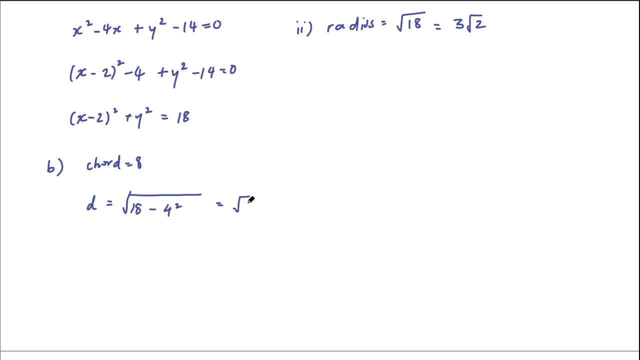 but let's finish this off. so this is 18, take 16, which will be square root 2.. so just to demonstrate why that works, if you have a circle and let's say the center, i'll try to draw the center, that's the center. then we have a chord. any chord, the shortest. 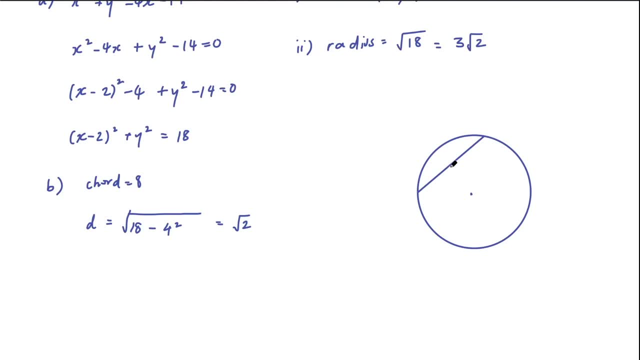 distance from the center to the chord is perpendicular to that chord, so that's meant to be 90 degrees, and so you create a right angle triangle, the radius being the hypotenuse, and the length we're looking for is one leg. the other leg is half the chord length, so that's going to be. 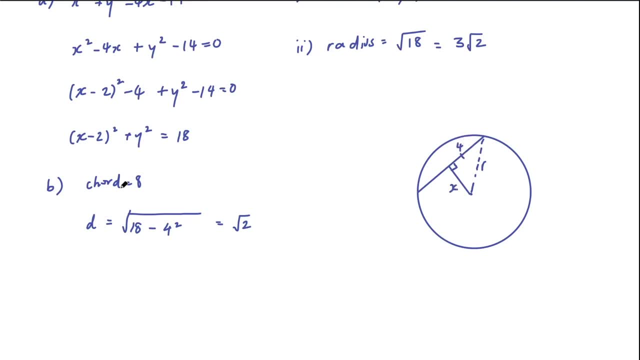 half the chord length, which is four in this case. so to work out the distance from the center to a chord, the shortest distance, you can always do the radius squared. sorry, the square root of the radius squared. take half the chord length, squared, okay. so square root two for part b. 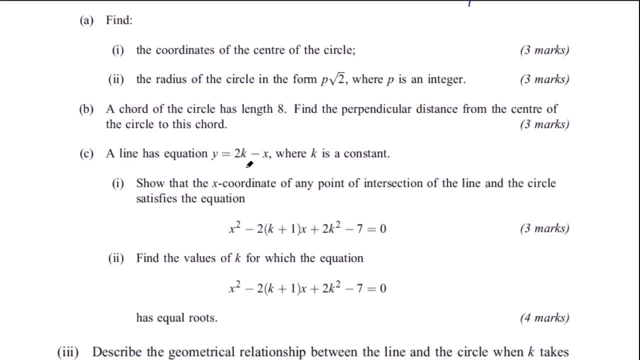 okay. so part c says a line has equation y equals 2k. take x where k is a constant. part one says: show that the x coordinate of any point of intersection of the line and the circle satisfies the equation x squared is equal to the radius of the chord length squared. 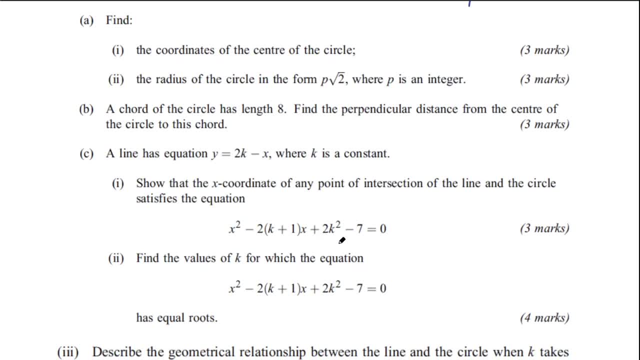 take two bracket k plus one x plus two k squared. take seven equals zero. all right, so when a line intersects the circle, the y coordinates would be equal and the x coordinates would be equal. so we could say the y coordinate of this line would equal the y coordinate of this circle. here. 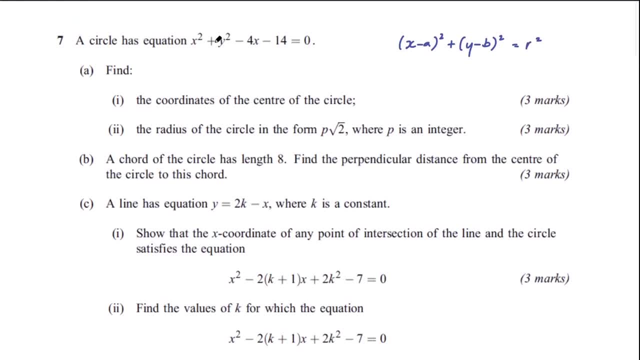 this is the equation of the circle. so when the y coordinates of those two equations are the same, we could effectively take this equation for the y coordinate here and substitute it into the equation for the circle, because when they intersect they're equal. so that's where we're. 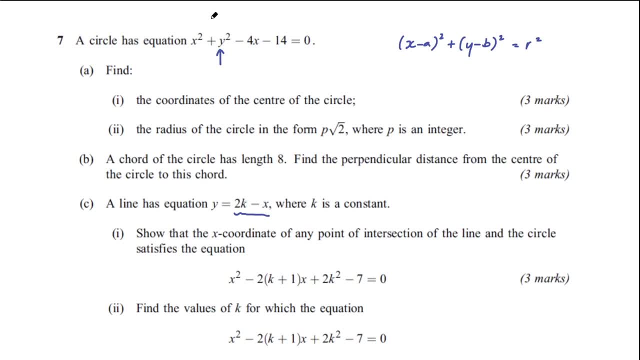 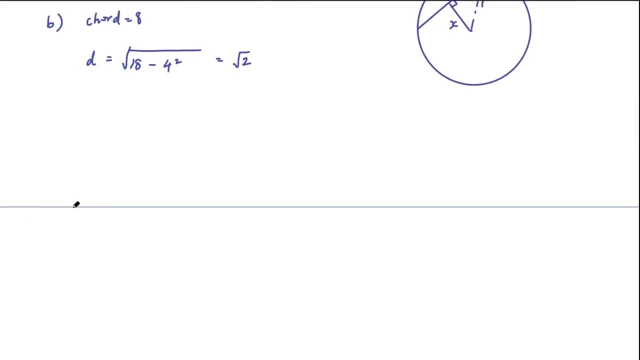 going to start. we're going to substitute this equation into the equation of the circle, because we're looking for when they intersect. so for part c, part one, i'll start that down here- uh, when the line and the circle intersect, we'll have, uh, the equation of the circle. 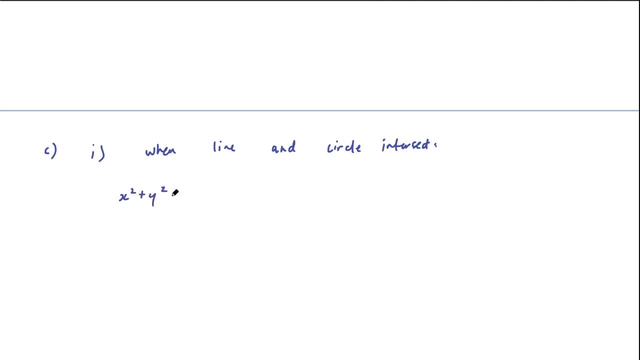 was: x squared plus y squared, take 4x, take 14, equals 0.. and the equation of the line was: y equals 2k, take x. and then we said: well, when they intersect, this y will equal this y. so therefore, x squared plus plus 2k, take x all squared, take 4x. take 14 equals 0. so now we have an equation in terms of x. 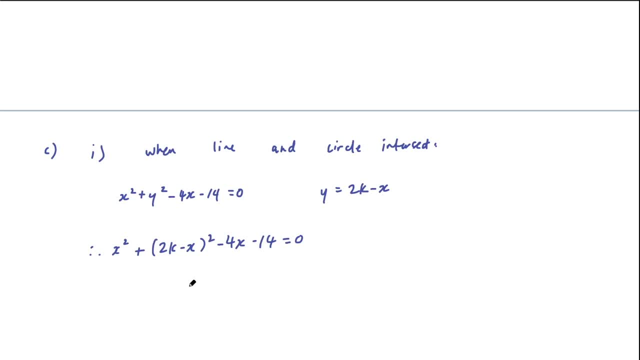 and if we solved this, we would have the x coordinate as well for when they intersect. okay, so now we need to go ahead and simplify this. so x squared plus. now we want to expand these out: 4k squared, take 4k. x plus x squared. that's what we get if we expanded those out: take 4x, take 14. 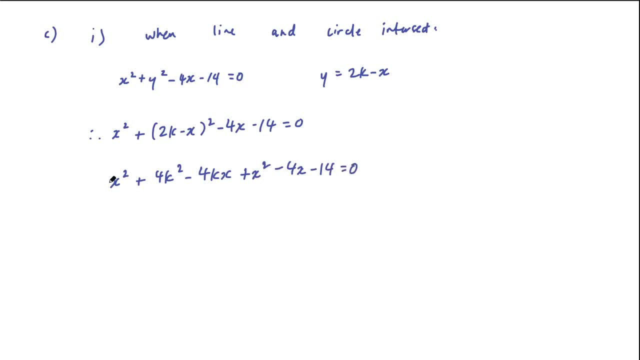 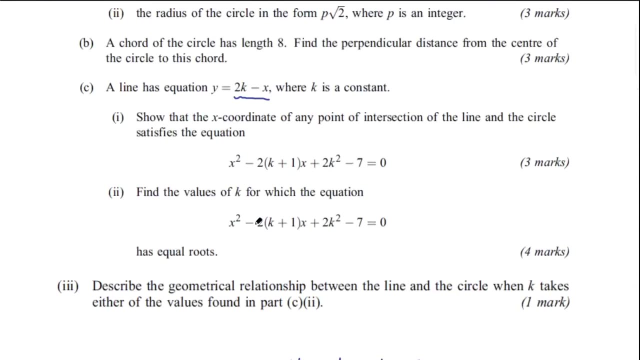 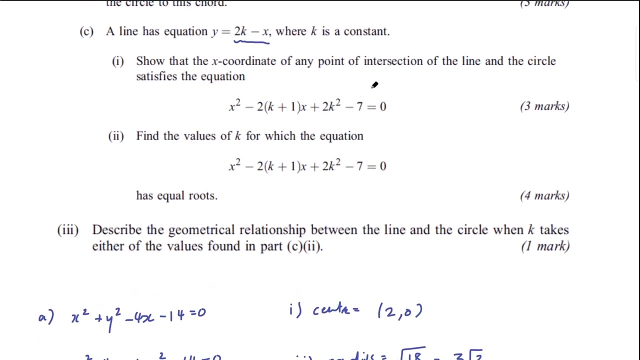 equals 0. let's keep simplifying: x squared plus x squared, 2x squared and that's everything i think we can simplify here. but if we go back to the question and just look at the form they have it, they have this k squared term towards the end, because these are the constant terms. effectively. 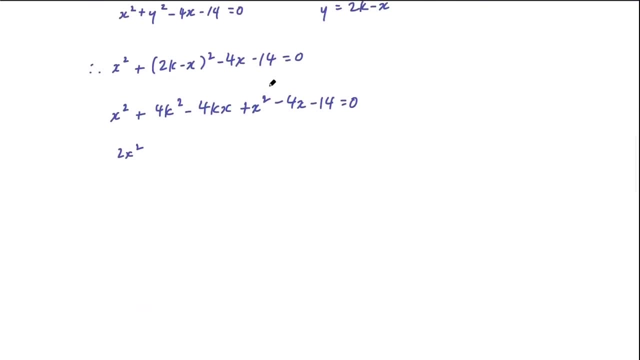 so let's combine the or write. write this slightly differently, so this would be negative: 4k- x. take 4x- they're like the middle terms of the quadratic- and then we have the constants on the end plus 4k squared. take 14 equals 0, then we could divide through by 2, so we have x squared. 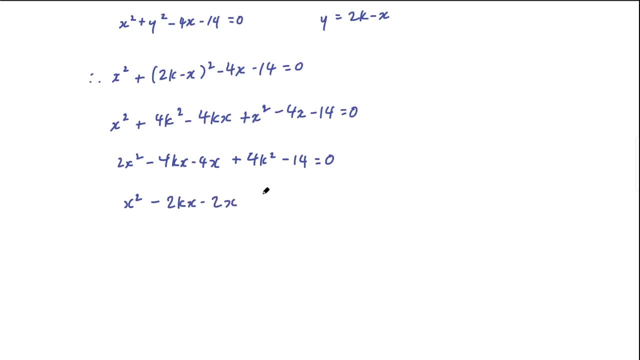 take 2k, x take, 2x plus 2k squared take, 7 equals 0. and then we want to factorize these middle terms here, so we would have x squared take, and i might do this in a couple of steps. so if we factorize, 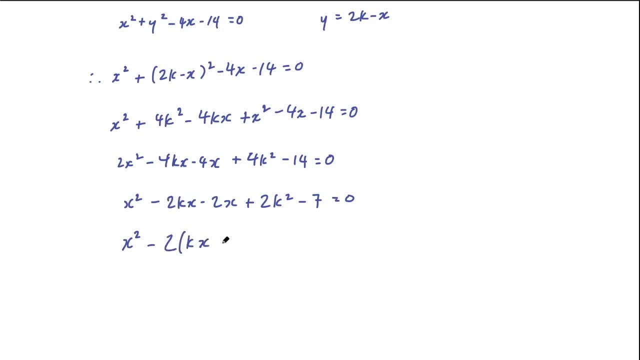 a negative 2 out, we would have kx plus x plus 2k squared. take 7 equals 0 and then factorize the x out, so we would have 2k squared. take 7 equals 0 and then factorize the x out, so we would have. 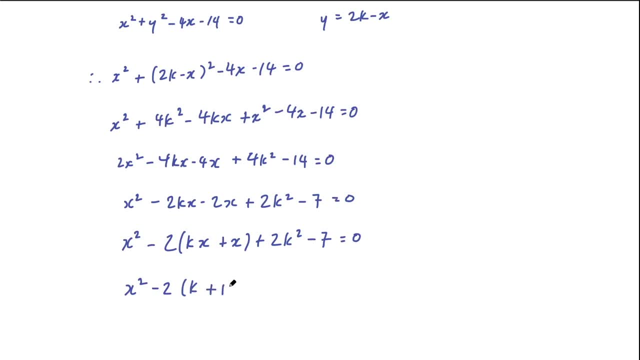 have x squared. take two k plus one. x plus two k squared, take seven equals zero. so rather than writing as negative two x k plus one, they write the x on this side as you would normally see it, like a normal quadratic right. so x squared plus ax or plus bx plus c, you'd have the constant before. 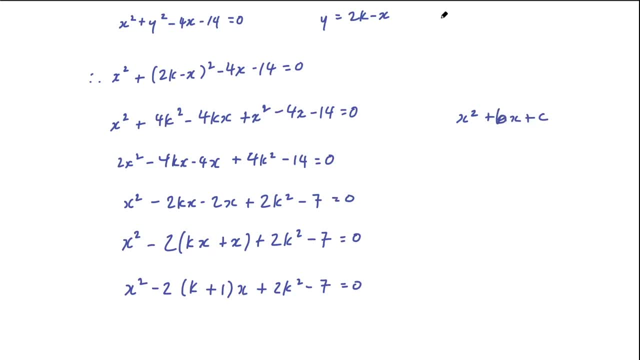 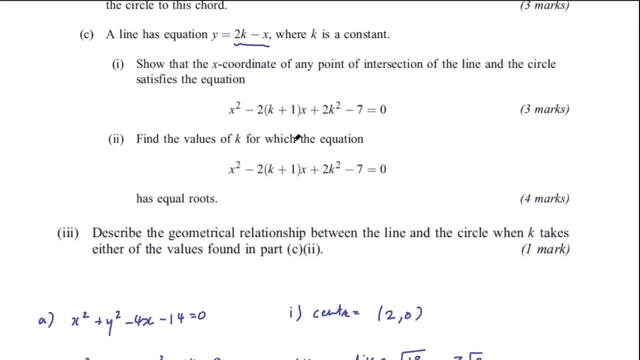 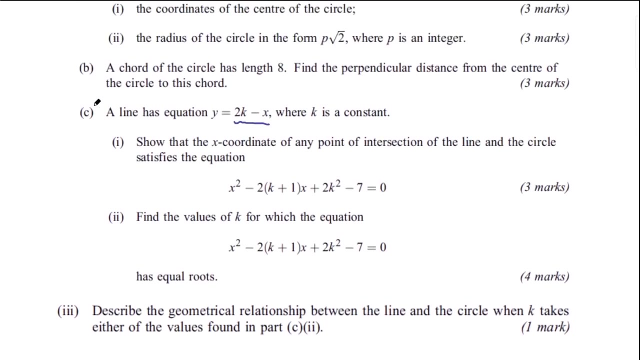 the x. so the x comes at the end there and and the constant before it. so that's why they've written it in in that form and then i think we have it in the form they're looking for. plus two k squared, take seven, yes. so there we go. that was question c, part one, and part two says: find the values of k. 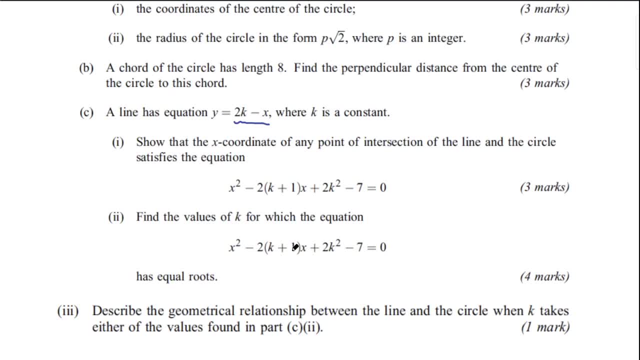 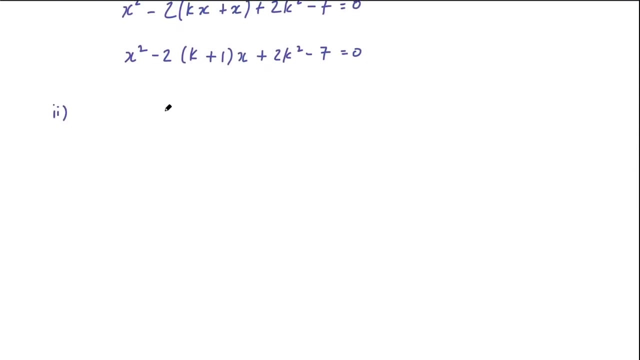 for which the equation x squared, take two k plus one. x plus two k squared, take seven, equals zero, has equal roots. all right, so i might just get started on part two and then point a few things out. so this is part one, okay, so there's little chance of being able to factorize this, so we're going to. 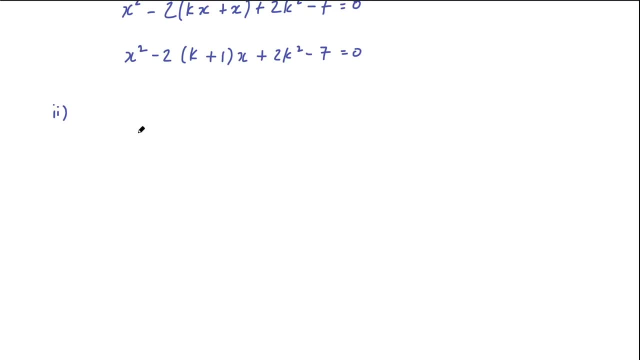 have to think about the quadratic formula and then the discriminant. so there are three different outcomes from the discriminant. you can have the discriminant, you can have the discriminant greater than zero and then you have two real roots. you can have the discriminant equal to zero and then you have one solution and then you can have 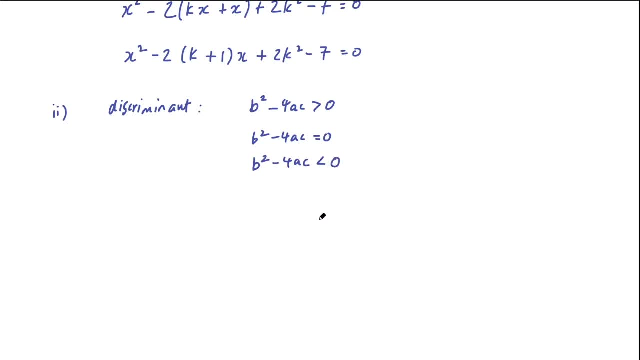 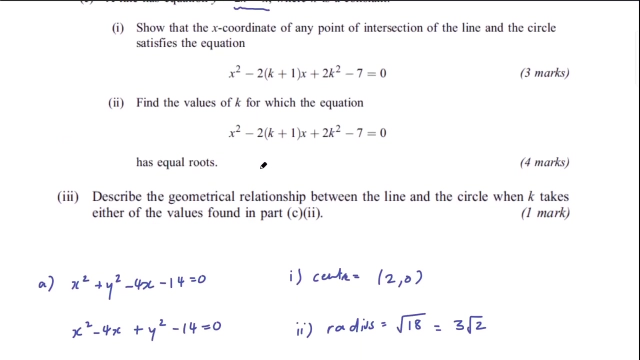 the discriminant less than zero and you have two complex solutions. okay, so for this one- remember, they've asked us to find the solutions for k, where the- how did they word it again, let me just check- has equal roots. in other words, that's effectively saying it has one solution. so we want the value of 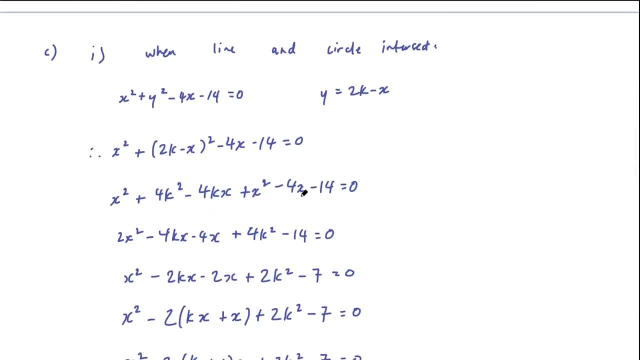 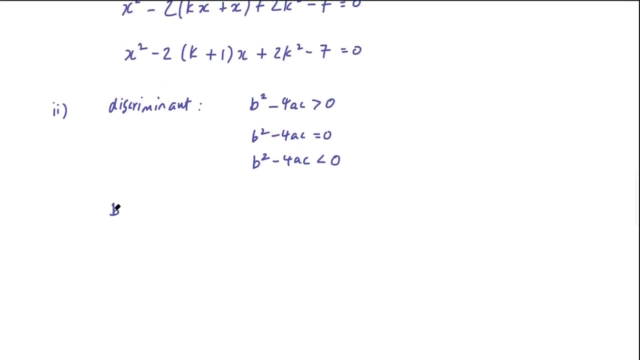 k for when this quadratic has one solution. so we, therefore, we want the discriminant to equal zero, um, so we can say that for the discriminant b squared, take 4ac for this quadratic. b is this term here, so let me just highlight or underline: so this is b and this is c right, because they 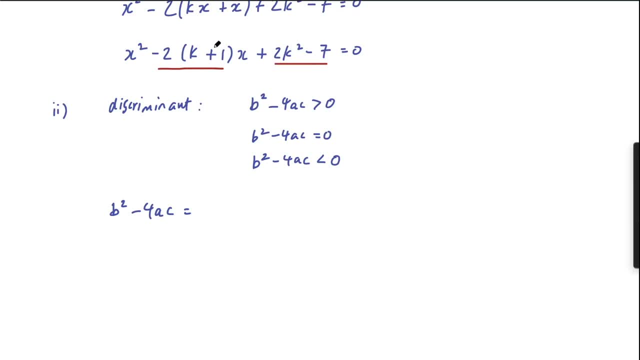 tell us k is a constant, so these are the constant terms. this is the of X, so B squared will be all of this squared, so we'll have negative 2, K plus 1 all squared and then take 4 times. a is just 1 and C is all of this, so C is 2, K squared takes 7. all right now. 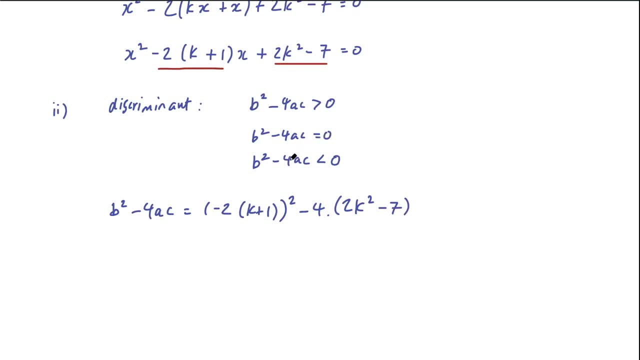 this needs to equal 0, to have one solution or to have equal roots- two ways of saying essentially the same thing. so therefore we can say: all of this equals 0, and I might simplify it as well. so therefore, negative 2 squared is 4, and then we'll have those brackets squared. so I've just 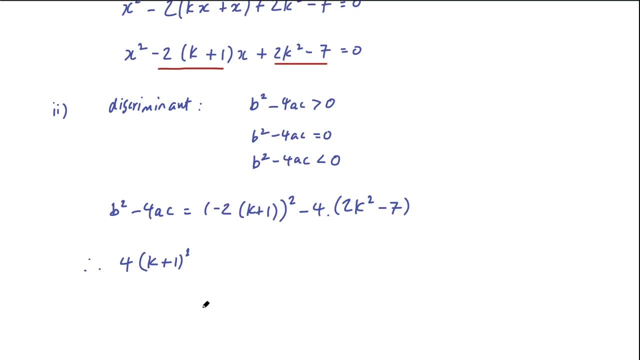 expanded that squared to both terms in those brackets and then we have negative 4, 2 K squared takes 7- I'll just leave that as is for now- and this equals 0. okay, now let's go ahead and simplify this. so if I expanded those brackets, 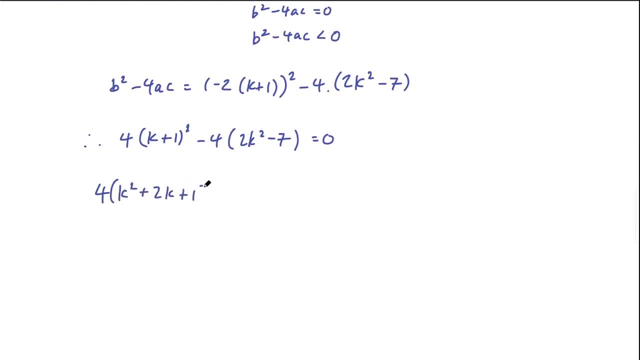 out, we'd have K squared plus 2, K plus 1, and then we'd have negative 8 K squared. take, sorry, plus 28 negative 4 times negative 7 equals 0, and then you could divide through by 4, so we would have K. 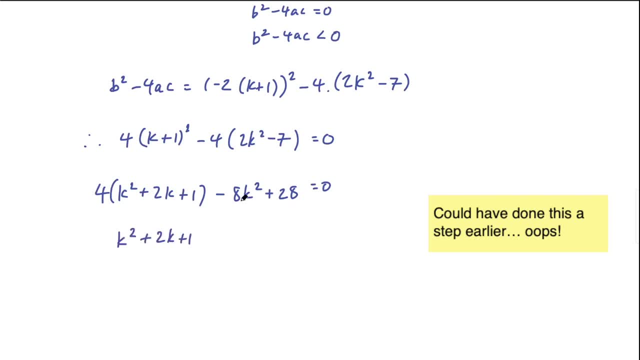 squared plus 2, K plus 1, because 4 is a factor of all of those terms. so we'd have negative. 2 K squared plus 7 equals 0, and then simplify further, so we would have K squared. take 2 K squared. negative K squared. 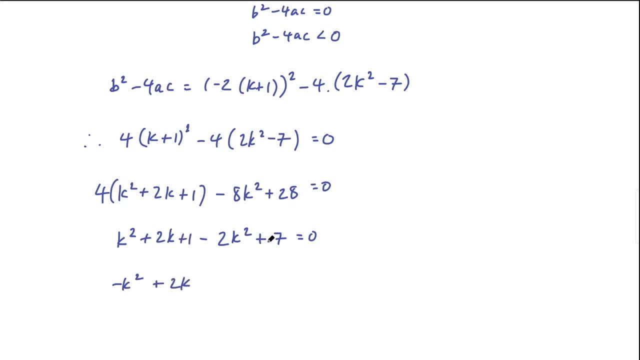 plus 2 K plus 1 plus 7 is plus 8, equals 0, and then I would divide through by negative 1, as I prefer to factorize when the squared term is a positive. so this would be negative 2 K, take 8. 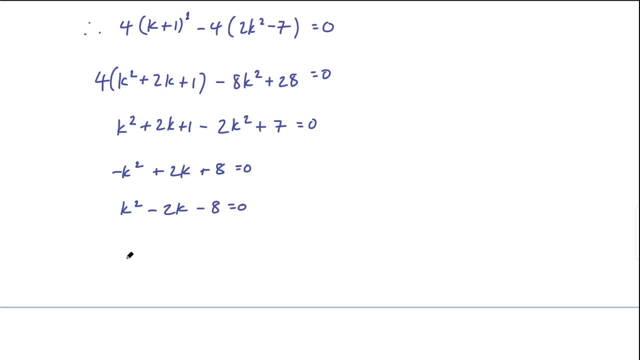 equals 0. then we have a quadratic. we can factorize factors of 8 to make 2, 4 and 2, and if that's a negative 4 and a plus 2, we'd get negative 2. so this would factorize to K. take 4 and K plus 2, so that should expand to K. 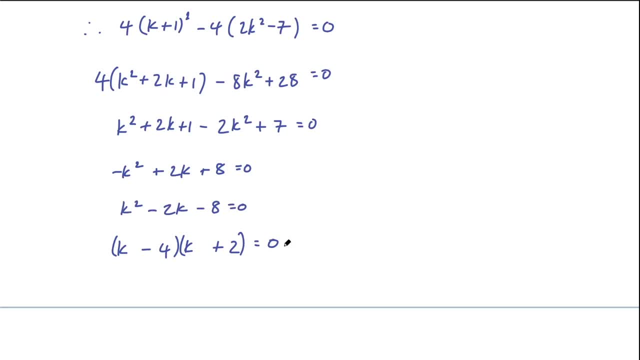 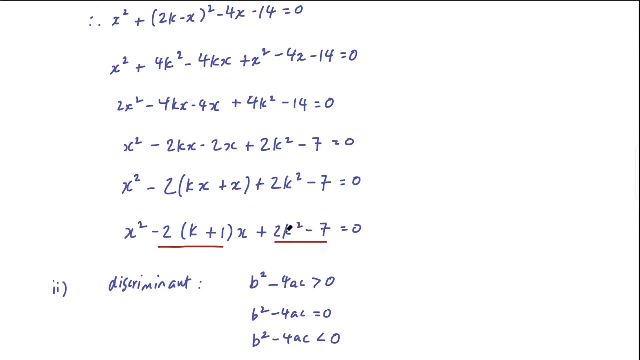 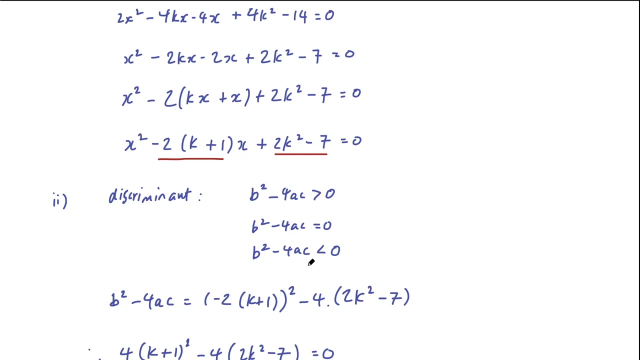 squared. take 2, K, take 8. okay, so now we have our solutions of K- K equals 4 and negative 2, and they are the solutions when this quadratic here has equal roots or one solution. so for that question you needed to understand the idea of the different ways, the discriminant. 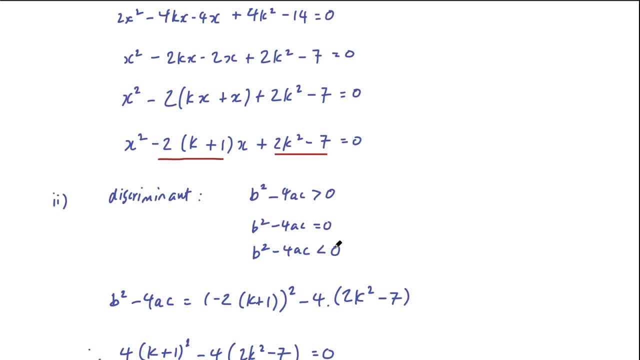 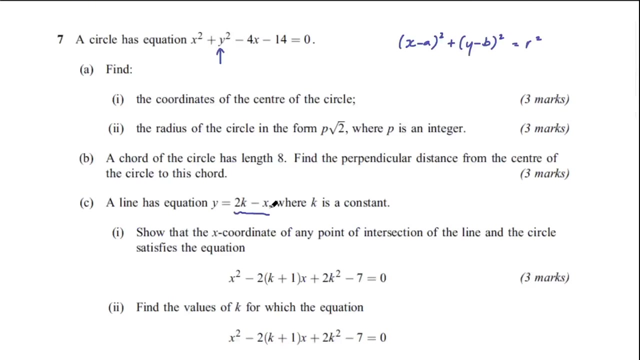 impacts the answer. so when it's greater than 0, when it's equal to 0 and when it's less than 0. so by understanding those three different types of answers, that really helps you with these types of solving quadratic questions where you have an unknown constant. alright, so that was part 2 C. part 2, part 3 says: 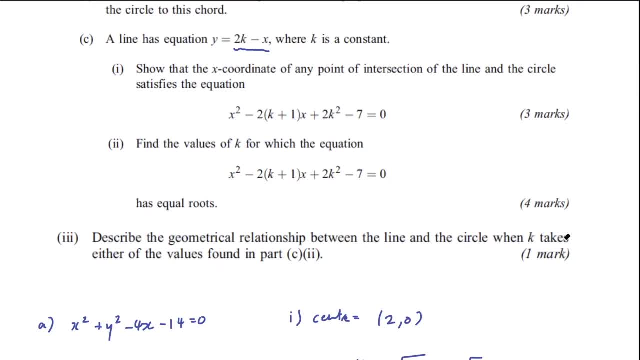 describe the geometrical relationship between the line and the circle, and K takes either of the values found in part C 2. here you really need to understand what you've been solving. so remember we got this quadratic by saying: this is where the line intersects with the circle. these are: 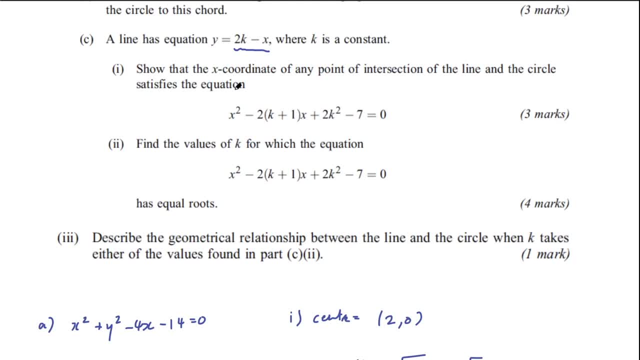 the x-coordinates for when the line intersects the circle. now, this is where the line intersects with the circle. so this is where the line intersects with the circle. so if we draw a circle, let's try to picture what's happening. we could have a line cutting this circle. 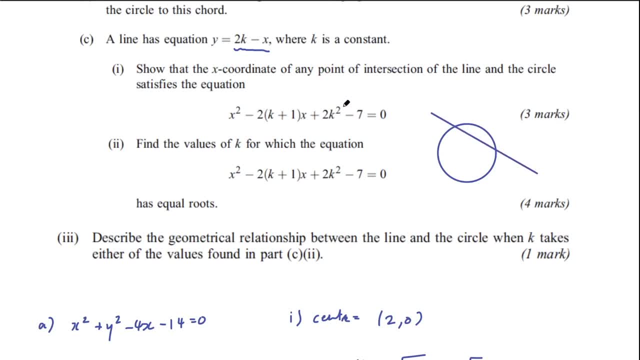 and if this quadratic had two solutions, it would cut the circle twice. then we would have two different x coordinates. now you could have a situation where the line would be vertical. then you would have the x coordinates being equal. however, we would have two different x-coordinates. 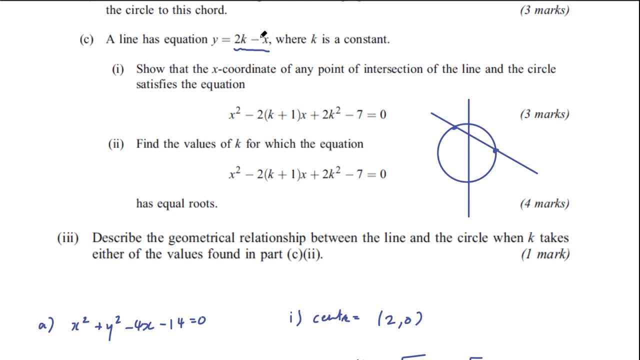 but we know this line is not vertical because the gradient is negative injured. so we essa uch, we know, we know this line is not vertical because the gradient is negative. we know that the we're not talking about vertical lines here. and we've said: for the values of K, the this quadratic has equal roots. so when K was four, cake was negative two it. 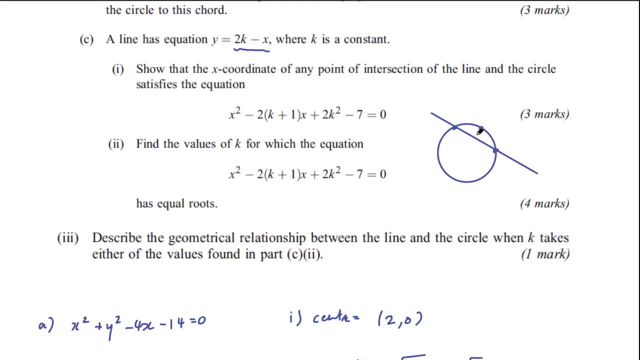 essentially had one solution. so that means that the line only touches the circle in one point. and what sort of line does that with a circle? that's the tangent line. so what's happening is when the circle when thes tangent line- right, so we're talking about tangents, when this equation has one solution.